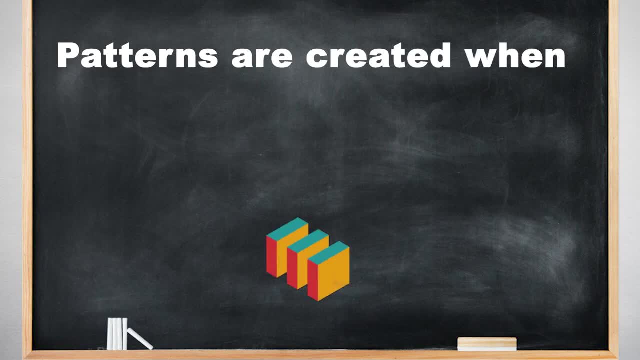 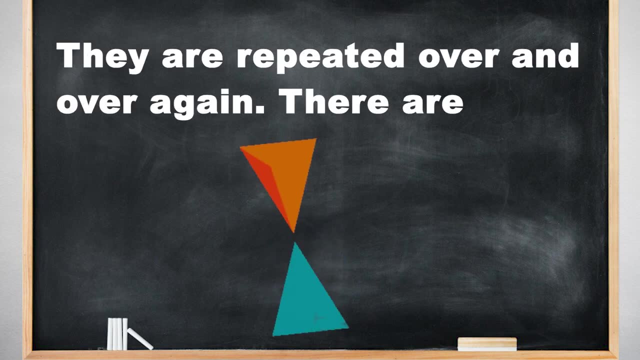 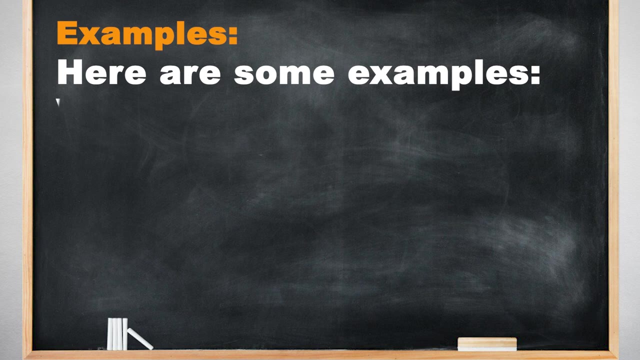 Let's go into it. Patterns are created when figures or shapes are arranged in a design. They are repeated over and over again. There are different types of patterns. Here are some examples, like rangoli, black and white stripes of zebra, bricks of wall Design is 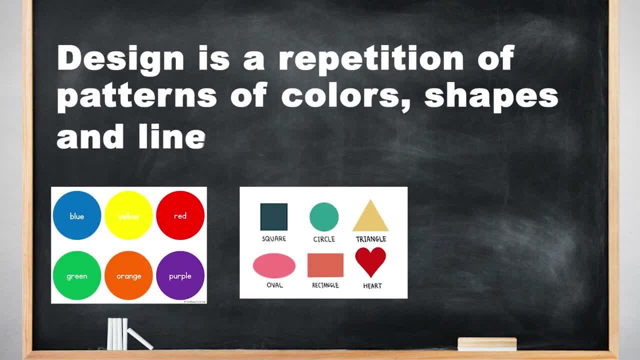 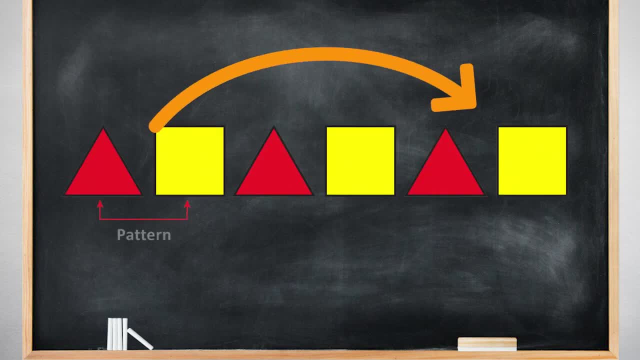 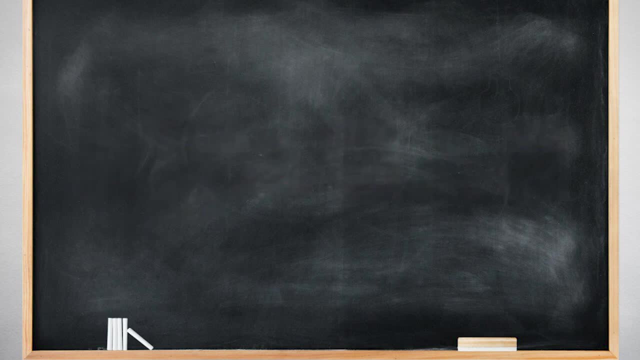 the repetition of patterns of colors, shapes and lines. Now that you know what patterns are, what is the pattern and design, check out the following design and observe the pattern. Can you see a red triangle followed by a yellow square, in repeat order It leads to the formation. 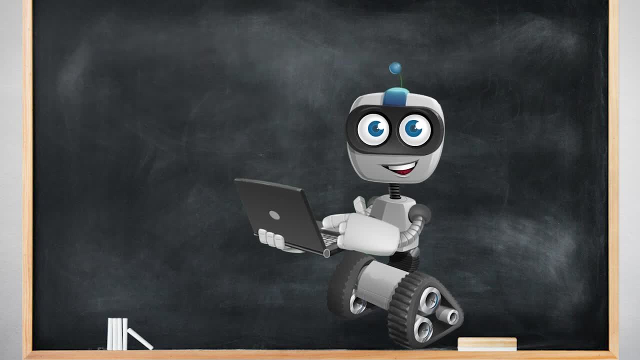 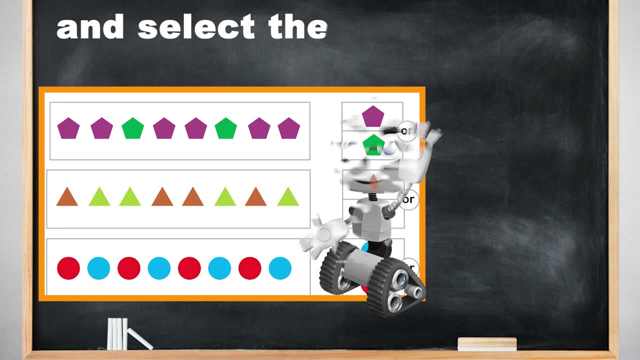 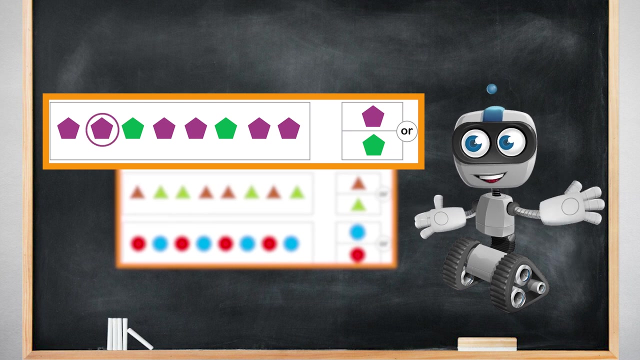 of pattern. Let's check out an activity For the first type of pattern question. look at the color pattern and select the correct color. The first is a purple pentagon, The second is a blue-purple pentagon, But the third is a green pentagon. This is followed. 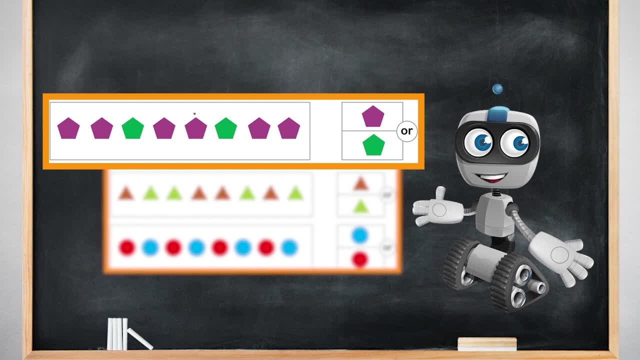 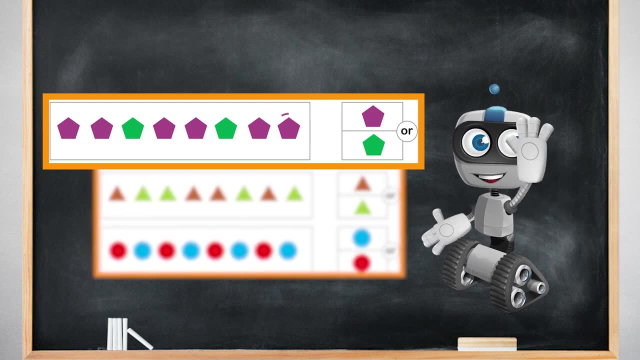 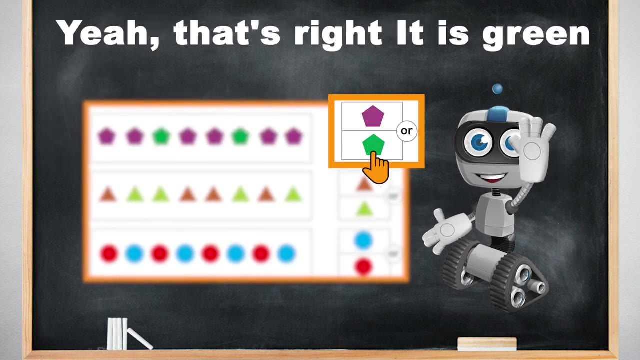 by another two purple pentagons. Now observe the complete pattern and tell me which pentagon will follow the two purple pentagons at the end. Is it the green one or the purple one? Yeah, that's right, It is a green pentagon. For the second pattern, question identify: 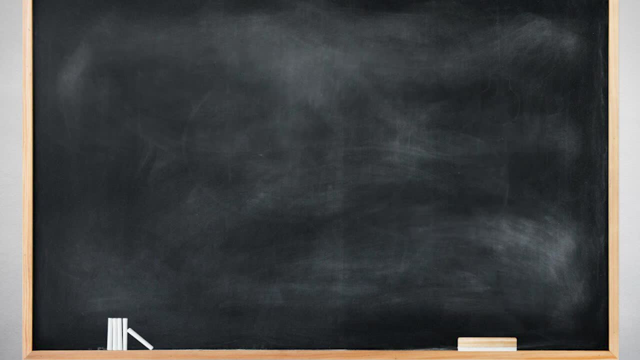 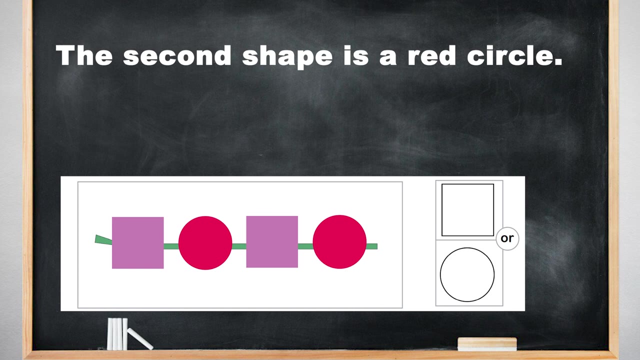 the shape pattern that comes next. The first shape is a purple square. The second shape is a red circle. The third shape is again a purple square. The fourth is a red circle. So what should the fifth shape be? Hmm, The correct answer is purple square. Good, 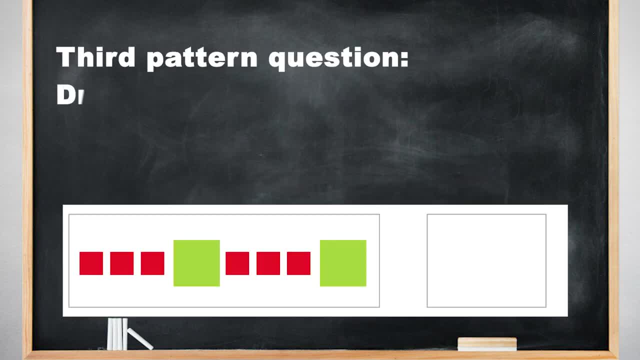 job kids. For the third type of pattern, draw the shape and size that comes next. Let us look at the question. The first three shapes are small red squares. The fourth is a big green square, followed by three small red squares and a green square. What do you think? 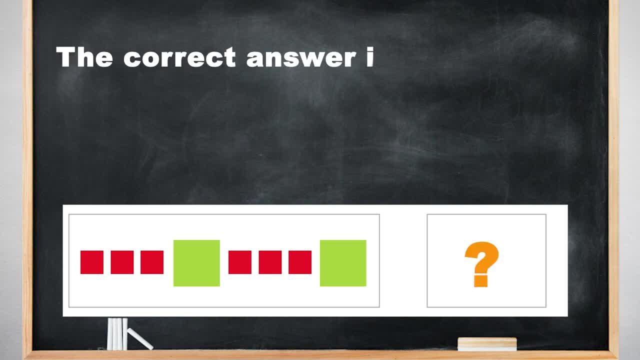 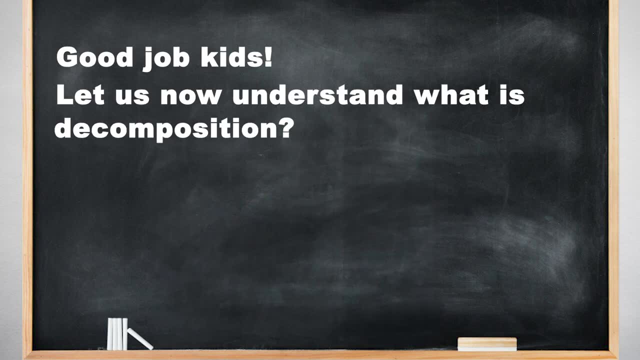 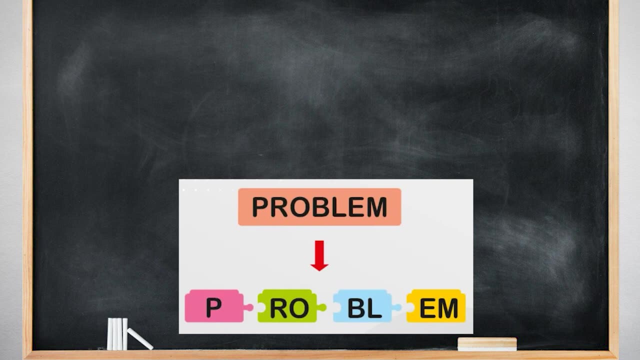 should come next? The correct answer is three small red squares. Good job, kids. Let us now understand what is decomposition. Decomposition means breaking up of a problem into smaller parts. Decomposition of a problem makes it easy to solve. Here we have a picture. 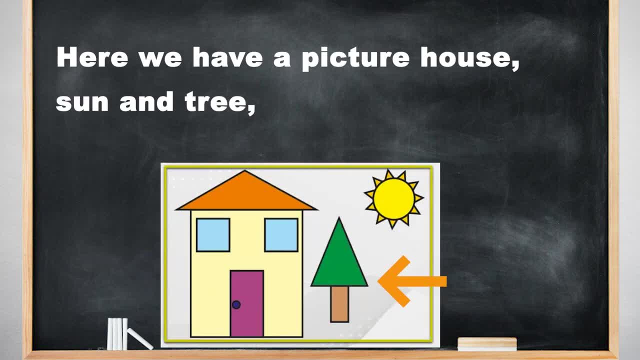 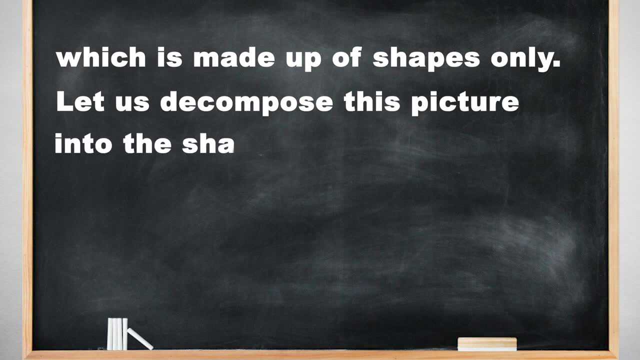 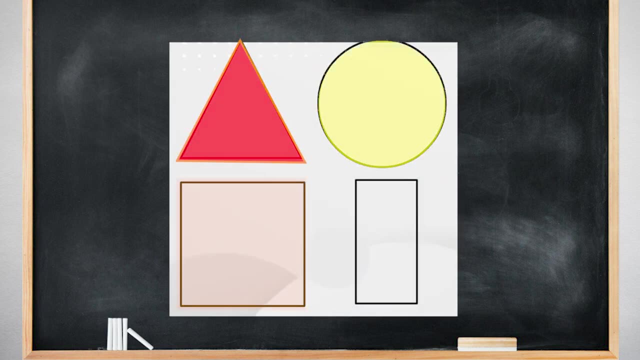 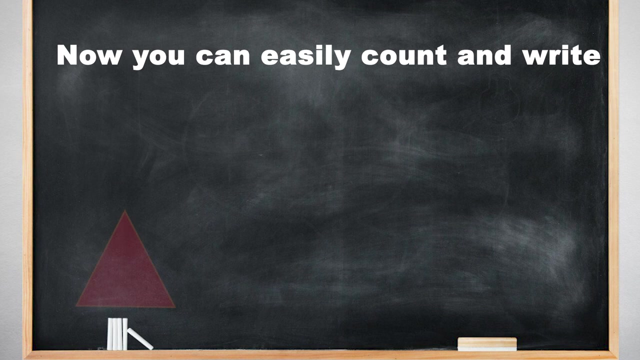 house, sun and tree, which is made up of shapes. only Let us decompose this picture into the shapes it is made up of. The picture can be decomposed into the following shapes: Triangle, circle, square and rectangle. Now you can easily count and write the numbers of the given shapes. It is easy to draw the. 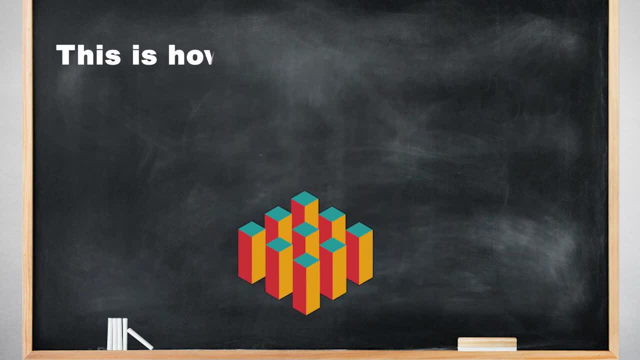 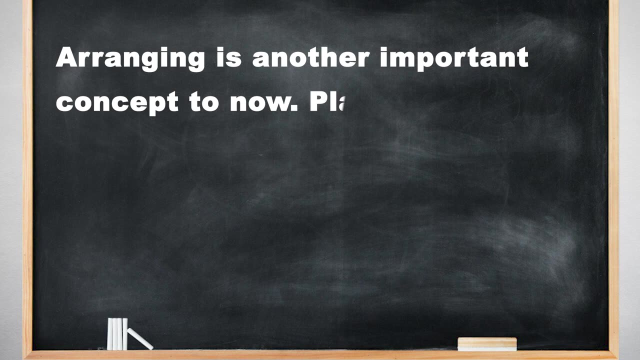 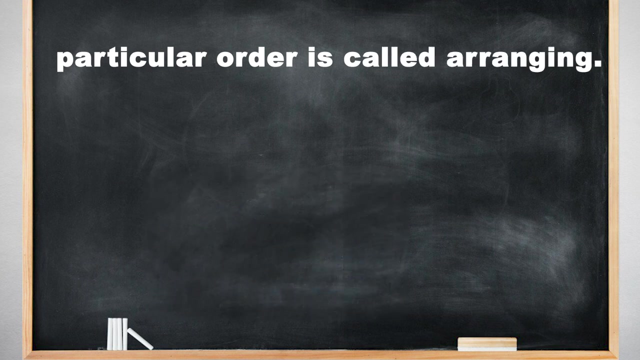 picture using these shapes. This is how decomposition helps us solve a problem. Arranging is another important concept to know. Placing a group of things at a proper point of the picture, at a proper place or in a particular order is called arranging. As you can see, everything. 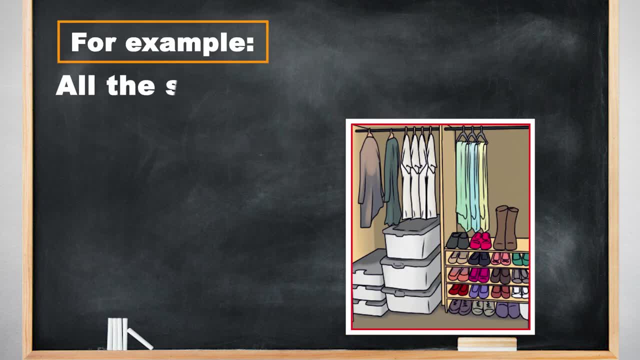 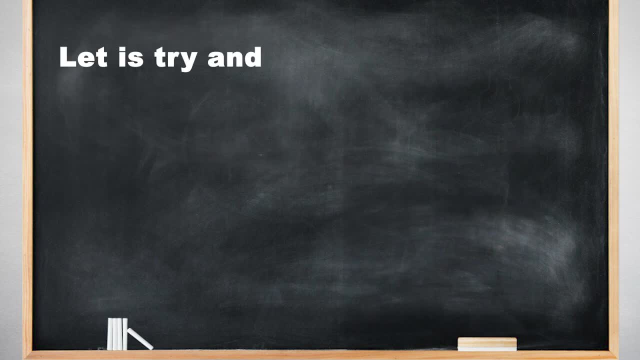 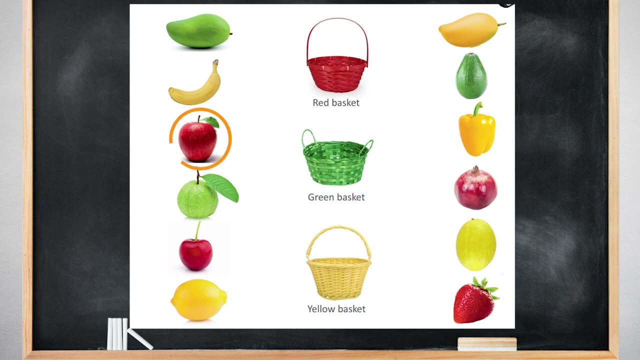 is kept in a proper order. For example, all the shoes are put at the bottom right corner and coats are hung on the left. Let us try and arrange the fruits with the baskets of same color. Where does the red apple go? Red basket, green basket or yellow basket? Let 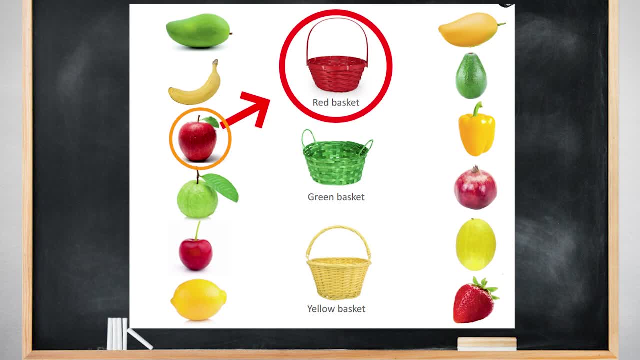 us try and arrange this trailing appreciate table. That's right, the red basket Because apple is of red color. Now where does the avocado go? Red basket, green basket or yellow basket? The correct answer is green basket Because avocado is of green color. where does? 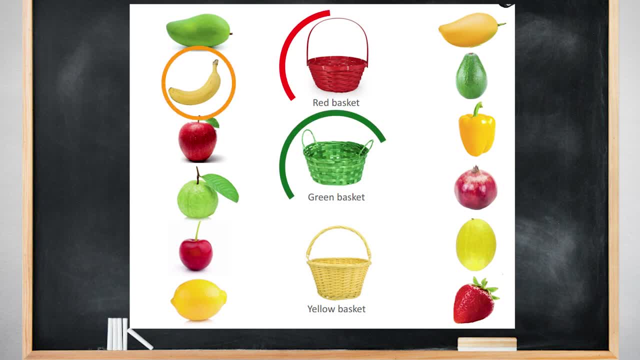 the banana go Red basket, green basket or yellow basket. Let us try and arrange this trailing heap. Let us try and arrange this trailing heap. Let us try and arrange this trailing yellow basket. That's right, Banana is yellow, so it will go into the yellow basket Now.